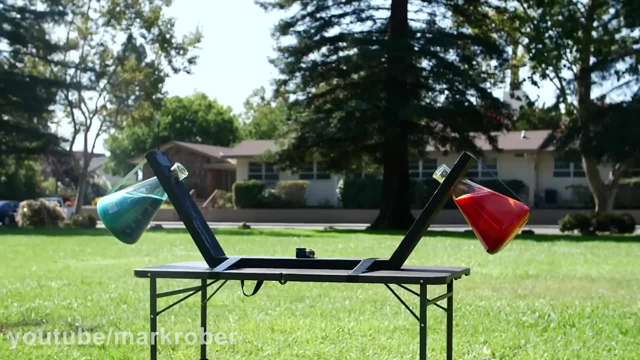 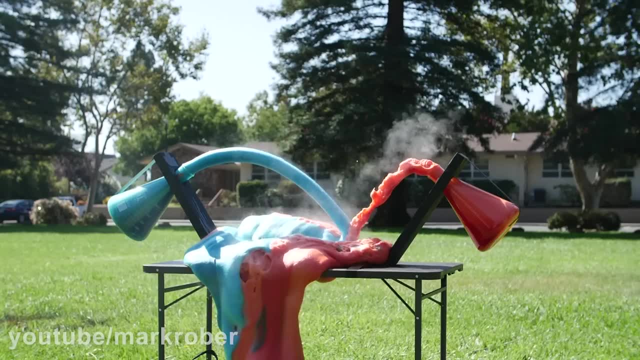 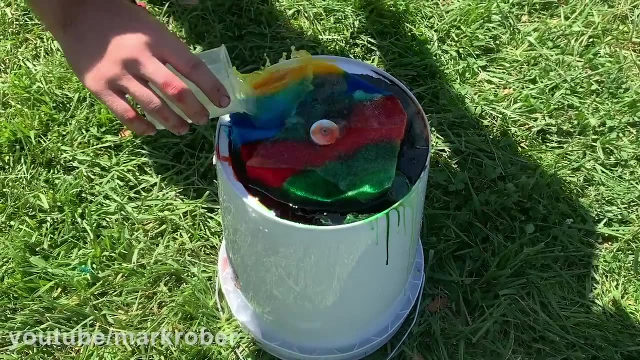 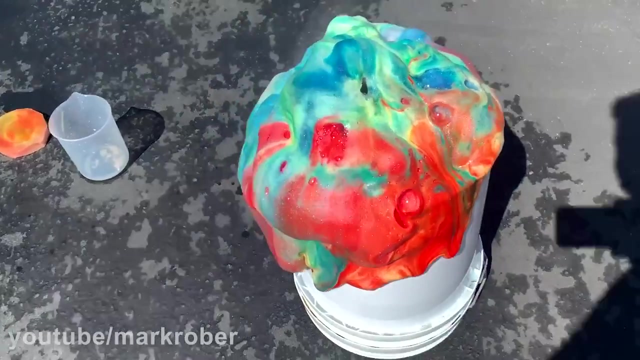 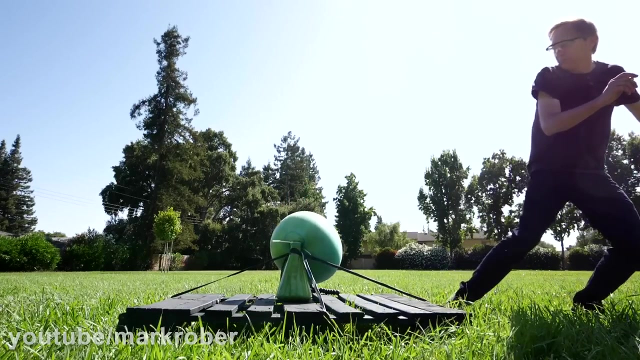 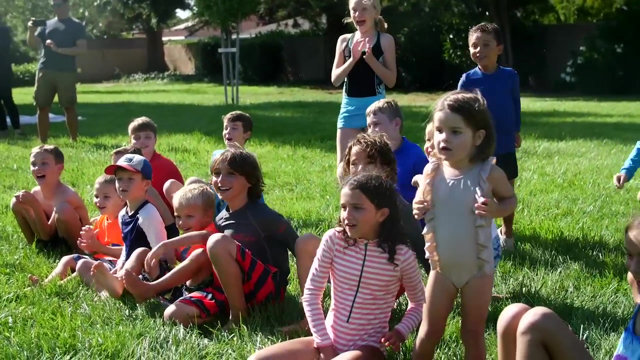 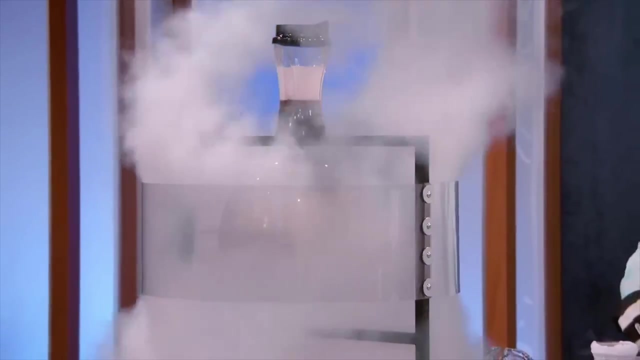 Three, two, one go. This one is called the melted unicorn. You might recognize Bob Flugfelder here, aka Science Bob. He's been on Jimmy Kimmel Live 11 more times than I have, and I invited him out to join me for a very specific reason, which I will address in a bit. 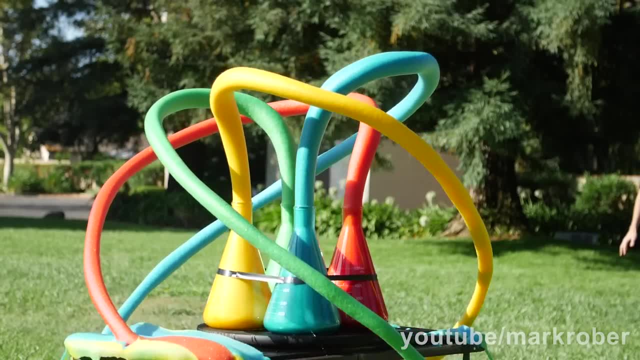 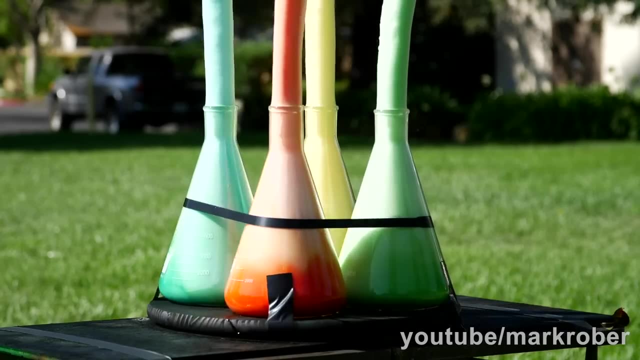 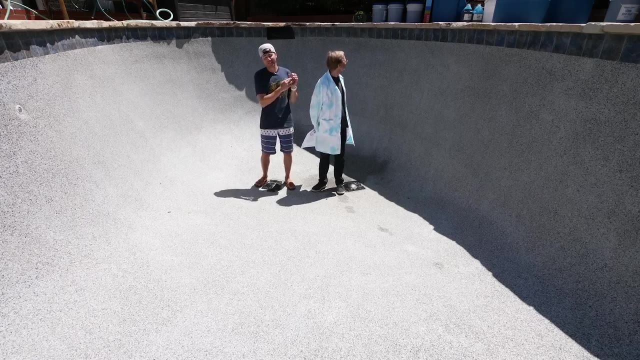 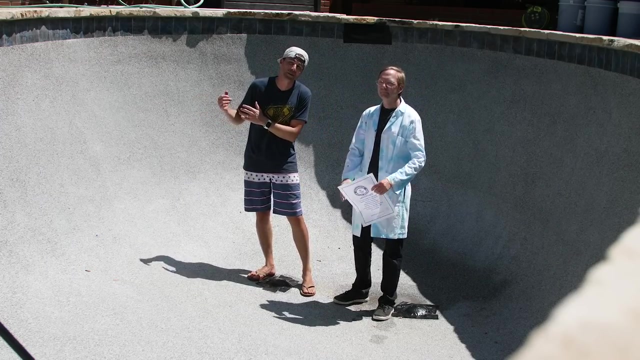 And so, with the success of the science show behind us, it was now time for phase two. So we are here, standing in an empty swimming pool about to try and break the world record for elephant's toothpaste. You want to tell the good people who owns the current world record, Bob? 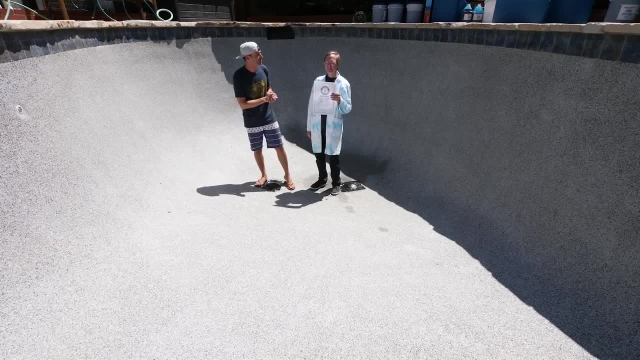 I do. You wanna tell the good people who's about to not own the world record, Bob, I'm pretty confident about that, aren't you? No, I'm not, Mr Engineer, But if everything goes well, we're hoping to quadruple. 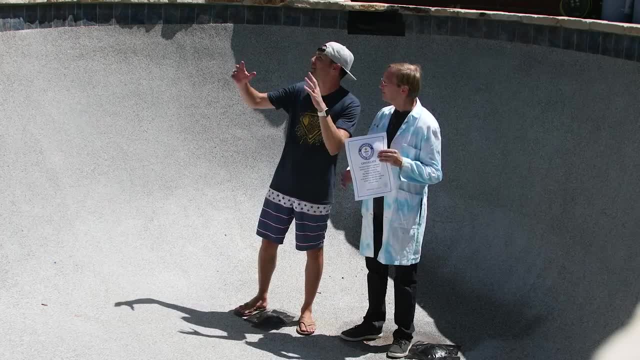 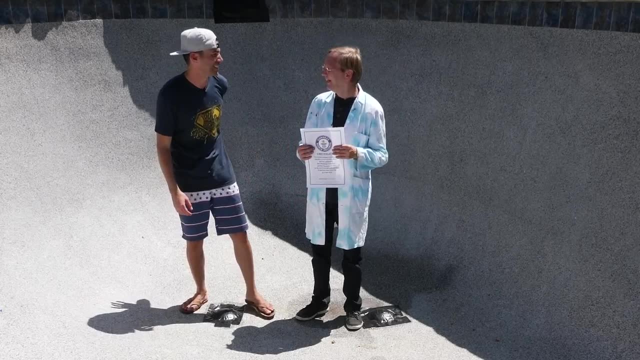 the amount of the current record which you hold. I'm not sure how much of like the trees and neighborhood we're going to cover in the process. Only time will tell- And chemistry which I don't understand, but we'll see what we can come up with. 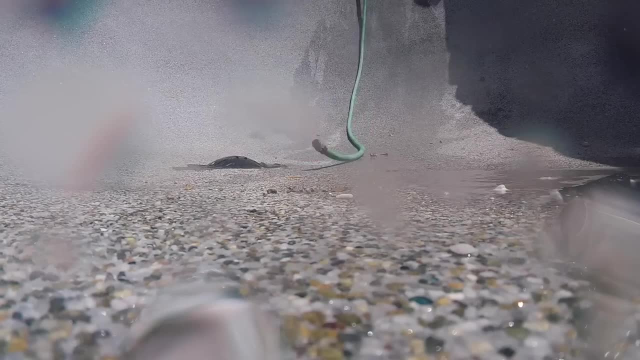 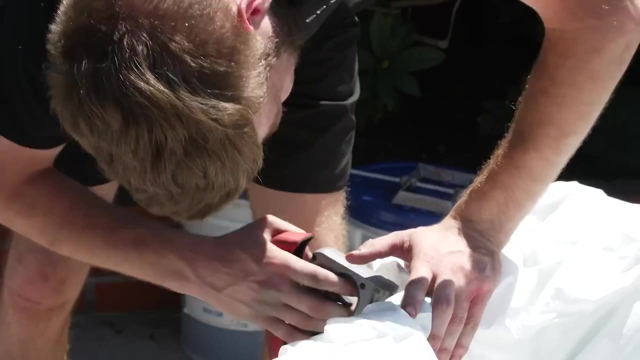 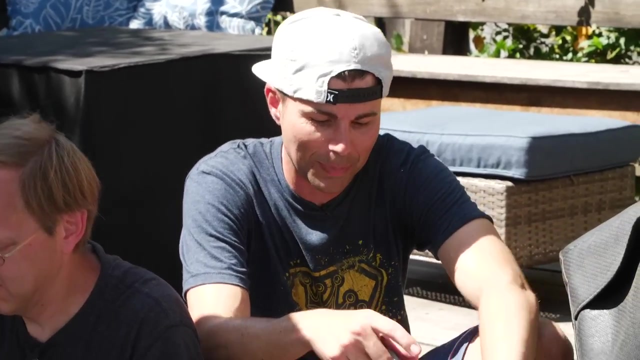 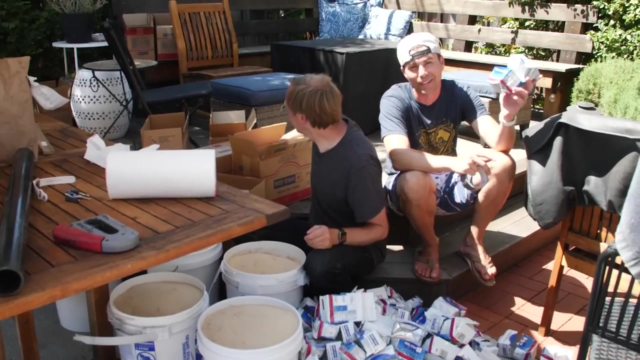 We wanted the phone to be safe to play in afterwards, so we used ordinary baking yeast as our catalyst. We could have bought yeast in big buckets, but it turned out it was cheaper to get them in one pound bags. The only downside to that is then you have to cut open 180 one pound. 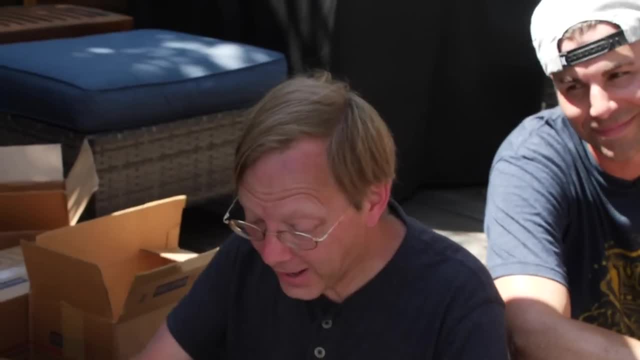 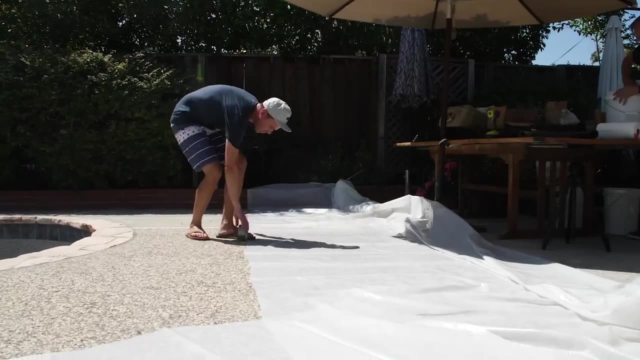 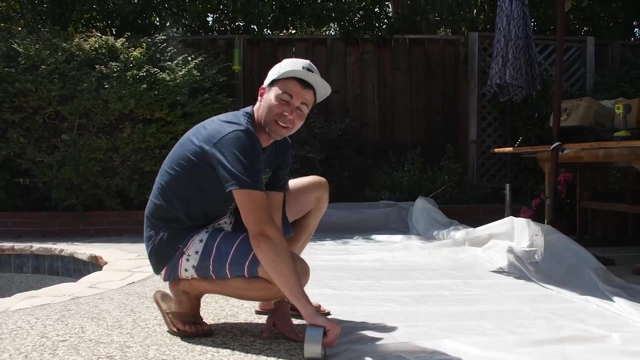 bags of yeast, But that's why we have Science Bob. Come on out. they say: This is an emergency tarp system, So if we did our math right, it shouldn't overflow. In the case that it does, we have these tarts here to contain all of the foam from not going. 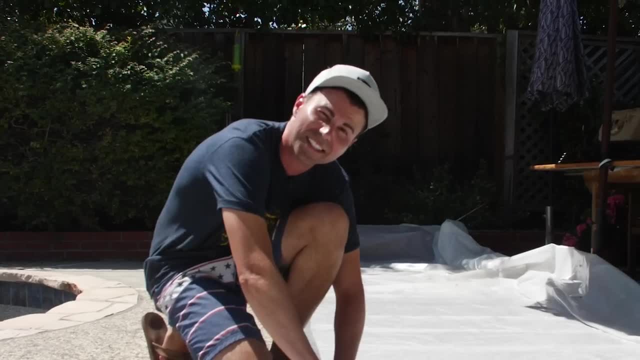 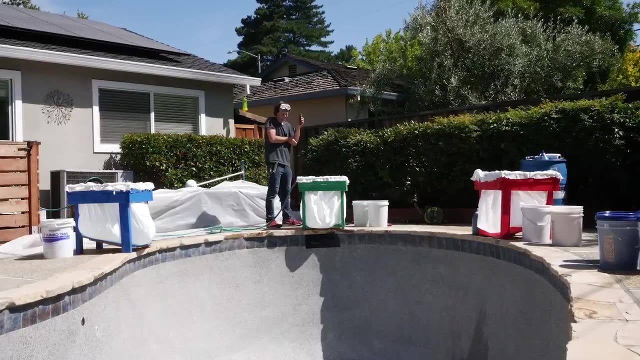 everywhere in the yard. We hope for the best plan for the worst. We built these three frames, We're going to put them in the oven and then we're going to make these frames for the tarps that would contain the catalyst yeast solution. So when? 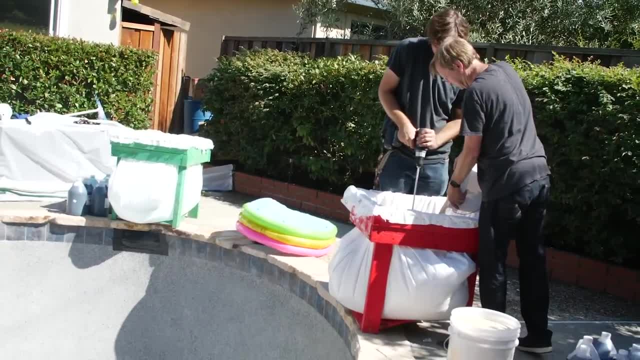 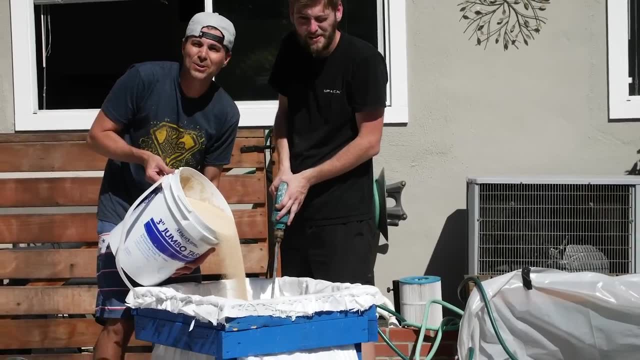 it was time to fill the pool. we could just cut the tarps and it would pour out, The same way we cut the tarp when we added the bigger Orbeez and Kevin. It's go time, baby. We're probably like seven minutes out, Got a bunch of kids inside. 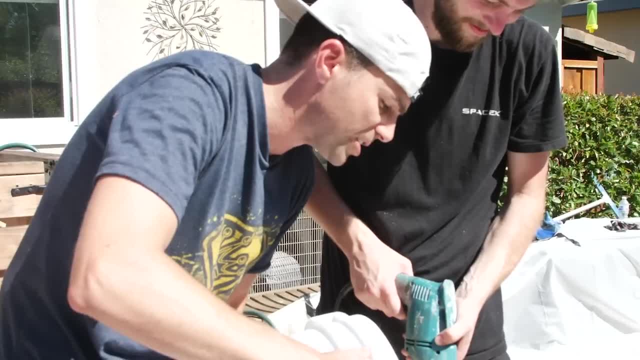 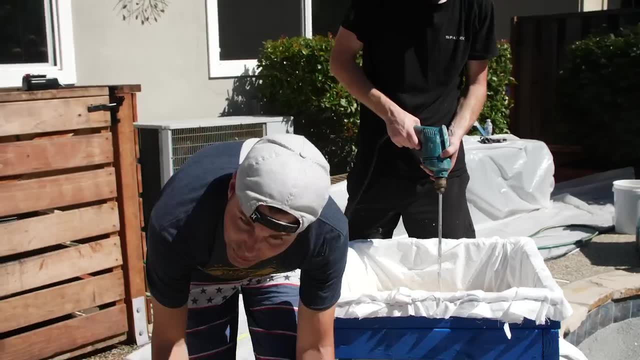 are just raring to get out. The challenge here is this water's warm. We didn't build these containers big enough, So this will start rising. It's sort of a racing race. It's going to be a little bit of a challenge. 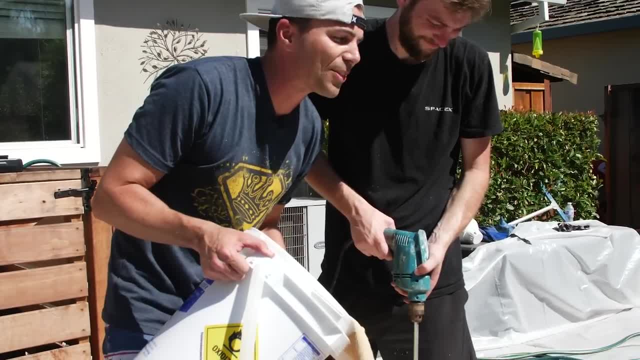 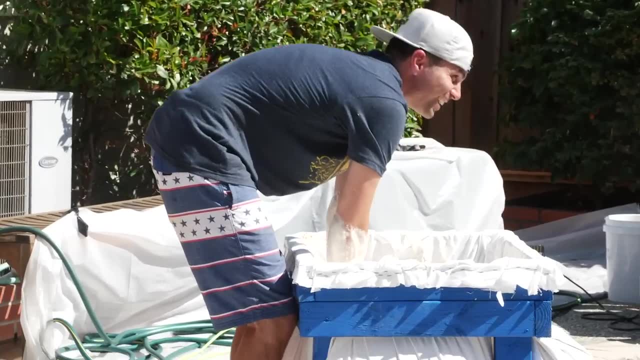 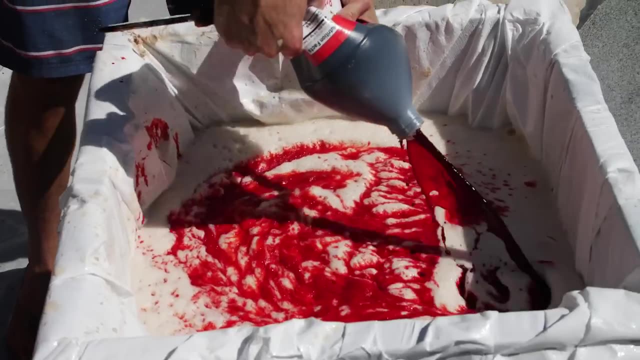 It's going to be a little bit of a challenge against the clock. before it starts overflowing, We still have to add the soap, and then we have to add the food coloring. Oh, this looks terrifying. as I stab this bloody thing, I think I'm about to get demonetized. 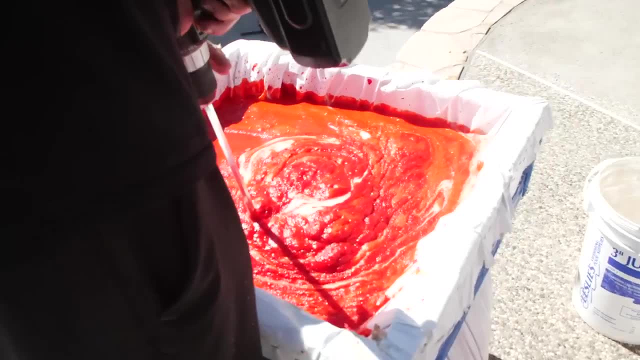 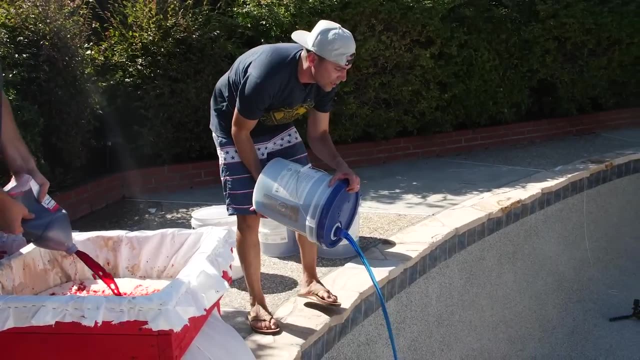 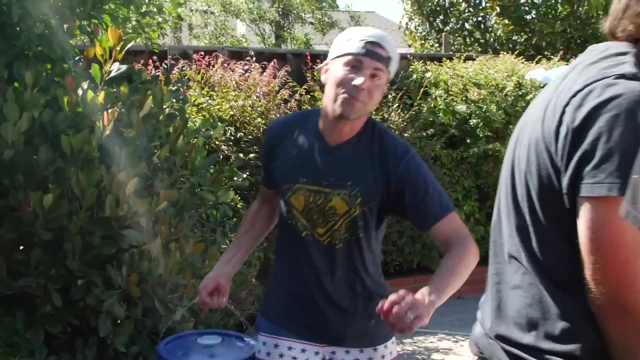 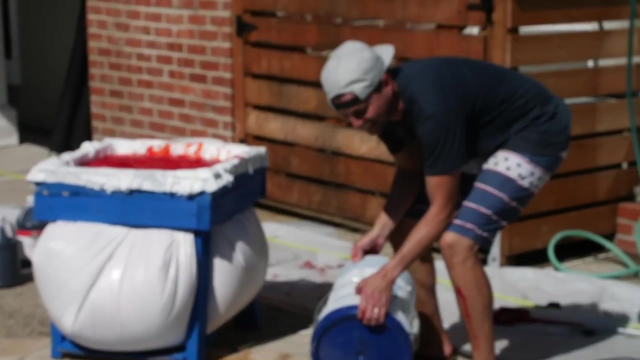 Okay, now we're adding the soap. This is what will actually make the bubbles. Soap isn't part of the reaction. Two more soap buckets. Oh, as you can see, that bucket's filling up real quick. So after a few final touches, we were ready to go. 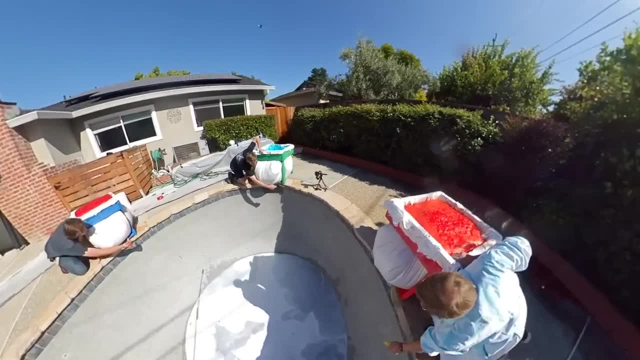 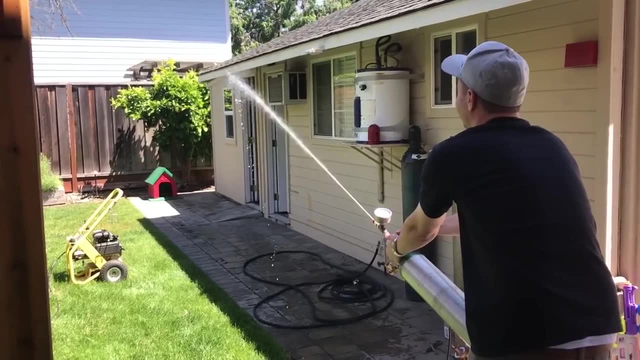 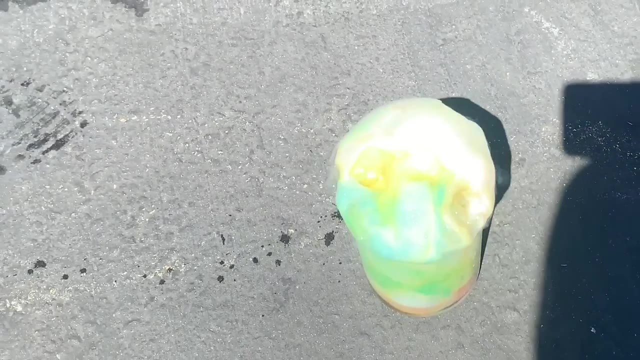 Three, two, one. Now, before we get the tarps, I want to point out I'm not a chemist. With the physics and engineering problem I'm way more comfortable understanding the parameters and getting closer to the final solution off the bat. But chemistry is just little molecules I can't see and it. 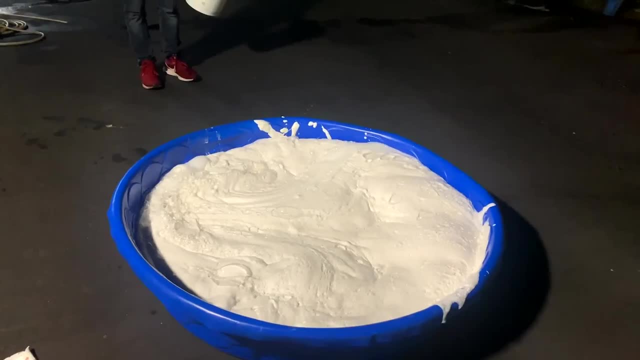 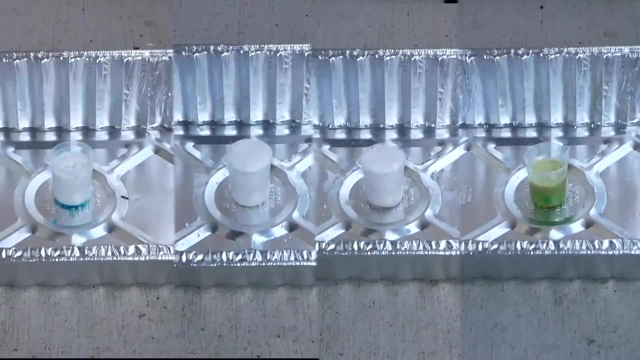 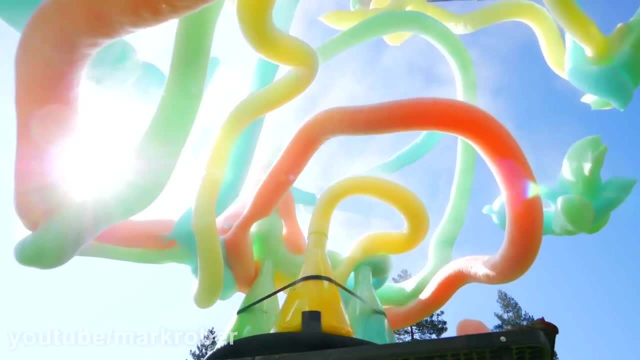 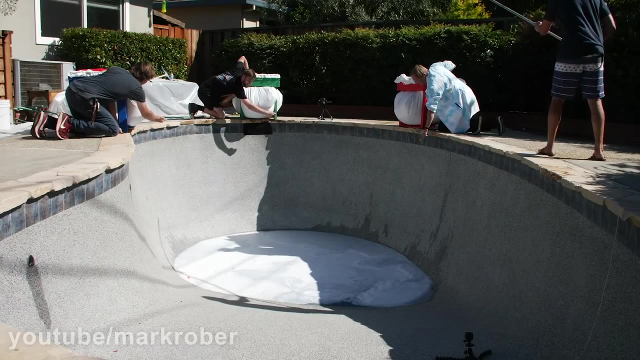 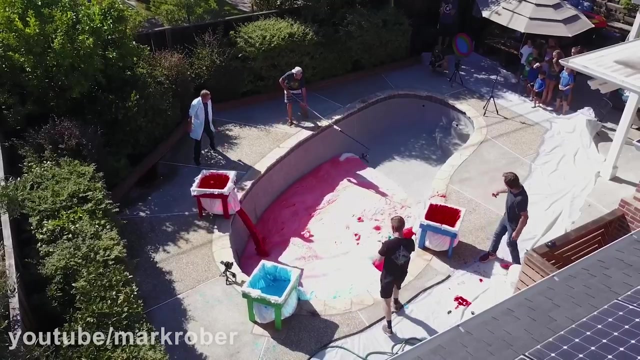 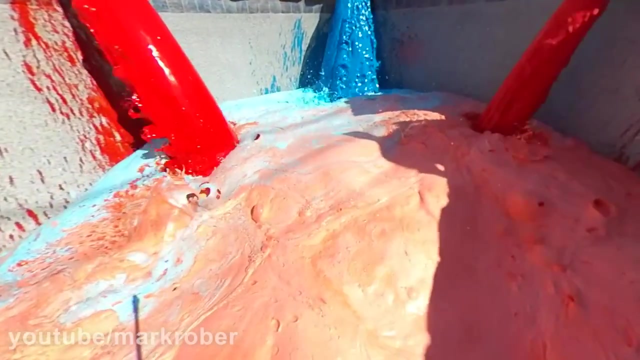 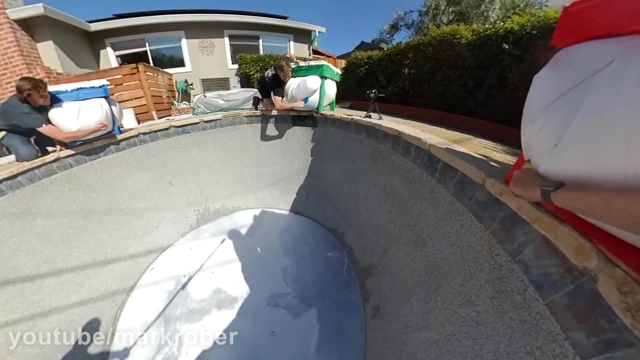 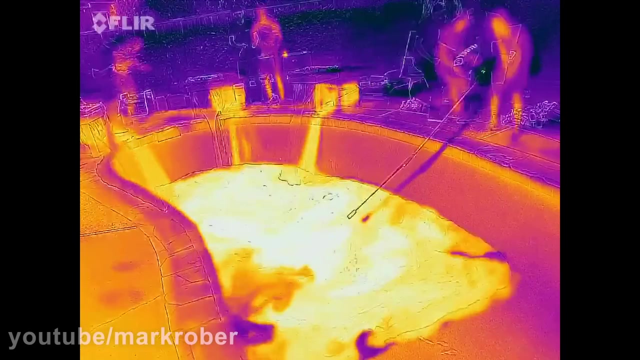 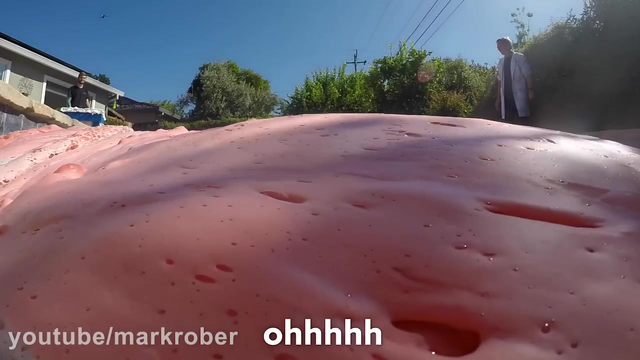 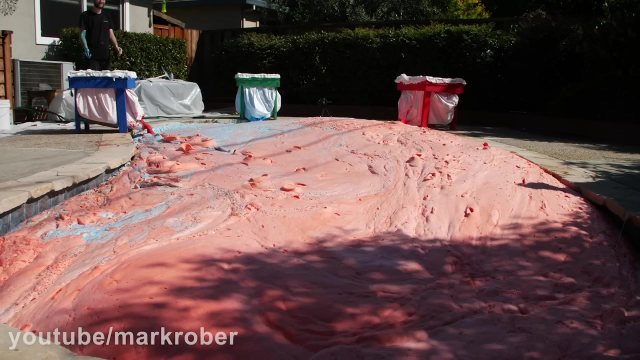 Great peril to that which we hold dear. And so, once again, if this was a total failure, it wouldn't be from lack of effort. Having said all that, here she is: Two, one go. so the good news is we broke the record. the bad news is we're kind of overachievers. 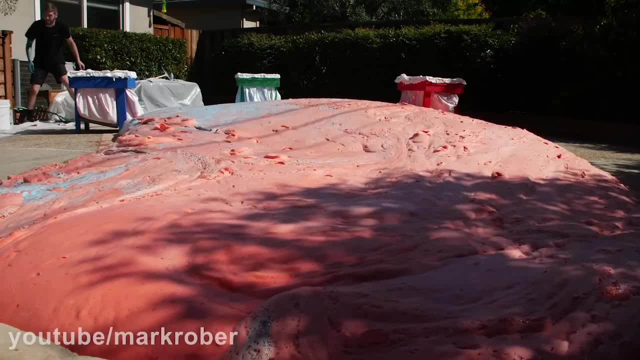 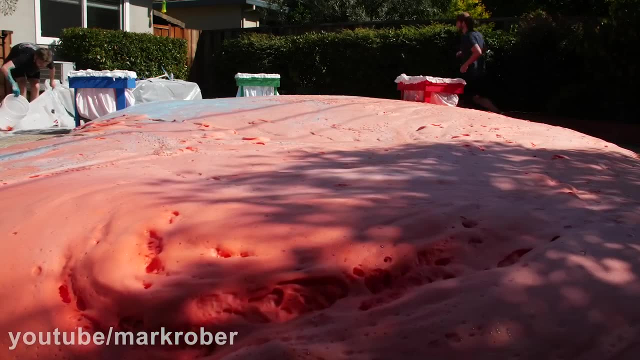 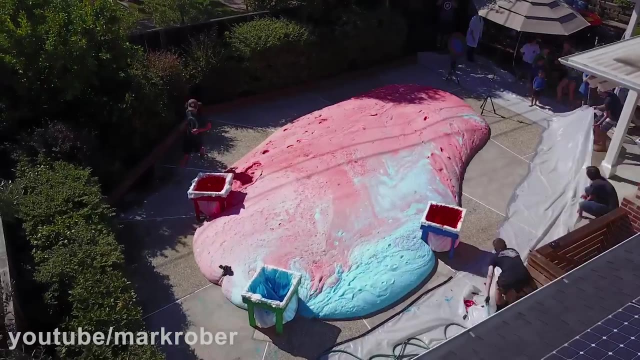 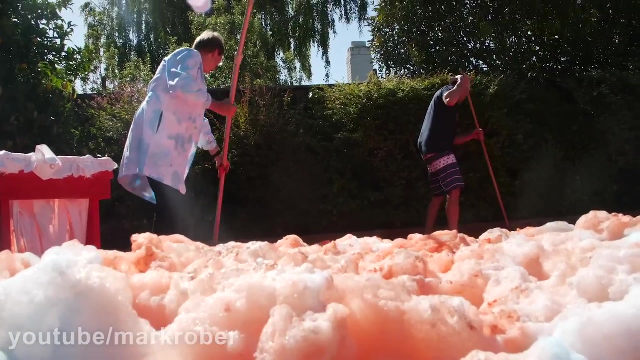 uh-oh, it's coming up, the great tsunami. hey, hold this okay. stand back off the tarp. oh, we need to grab them. stand back. hold this up, bob, okay. so while we pushed all the foam back into the pool, that gave it some time to cool down. 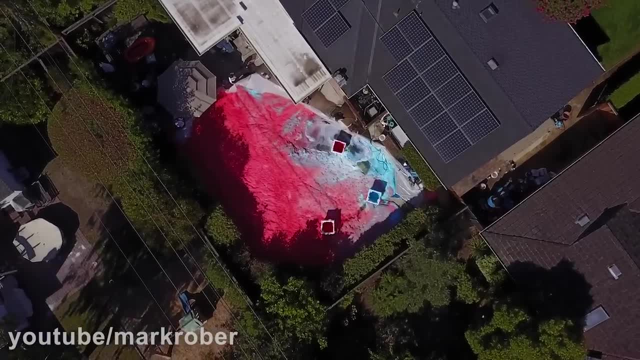 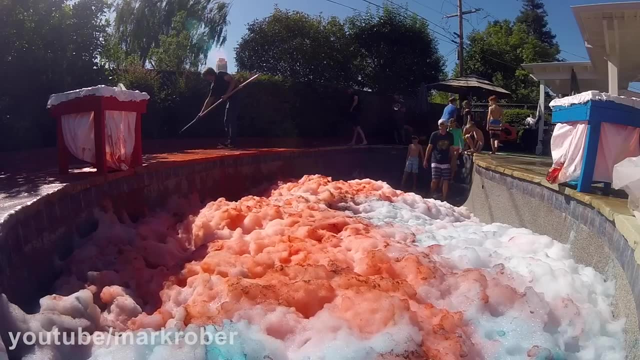 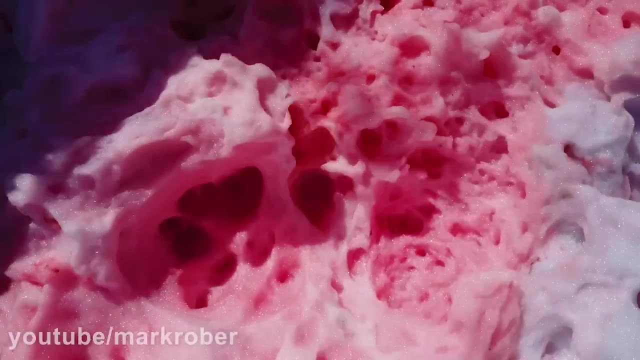 so we could actually touch it. the drone was super cool because not only did we get to see the sea, but we also got to see the ocean and the sea. not only did it make the foam look like an alien cocoon, but you could see it travel in. 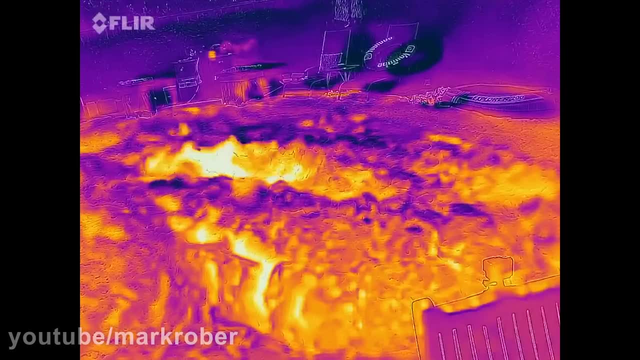 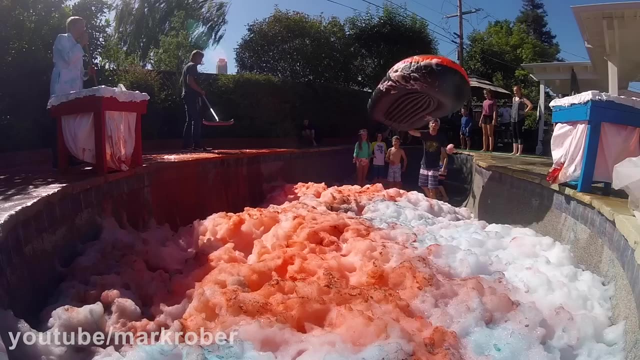 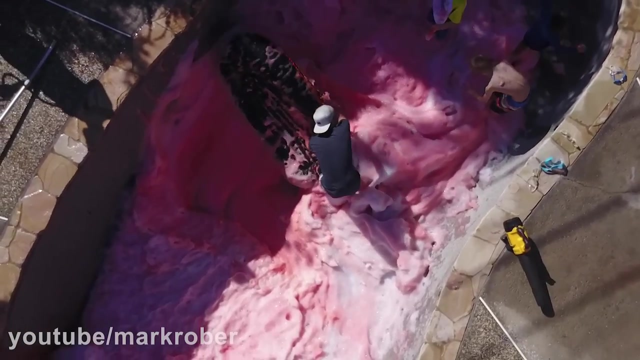 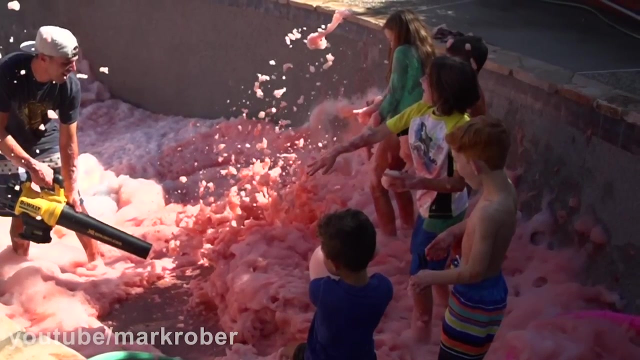 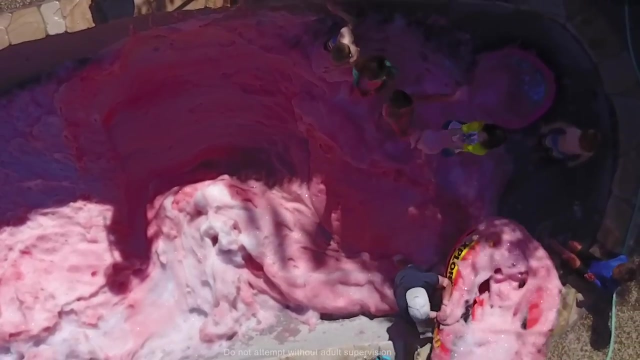 infrared, because it would expose the much hotter lower layers of foam as it flew around. what do you guys think? do you think this is gonna float? no, all right, here we go. it's gonna float. after all our tests, we perfected the chemistry for this stuff, so if you want to make a home version, you can play with. check out Science Bob's website. 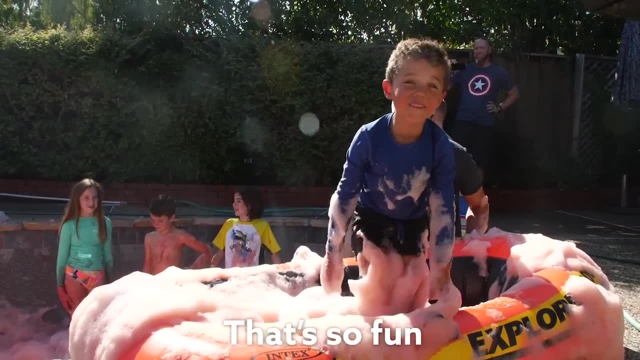 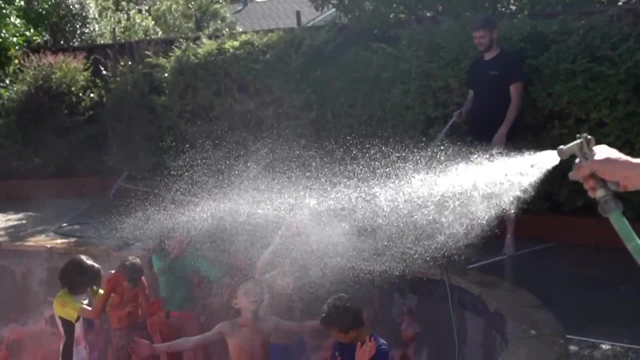 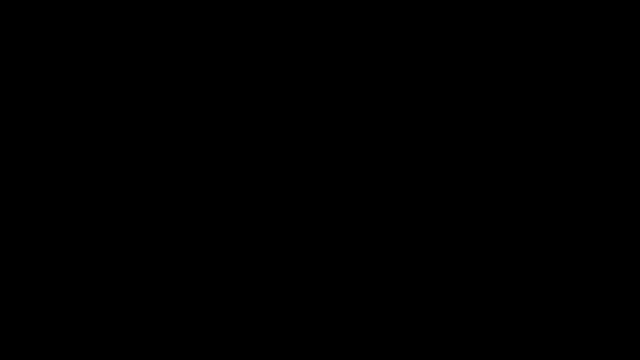 i'll leave a link in the video description. all right, Bob, sorry you're looking at an obsolete piece of material there before we anywhere now. hey, that's four feet away. THAT'S SO FINE. you've got to guard that so quick, don't you?